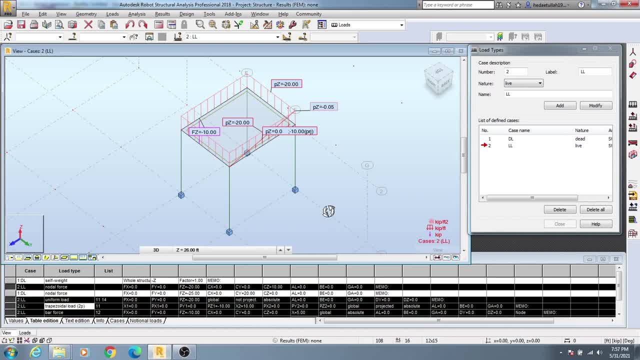 Hi, welcome back to Scrum, Civil Engineering. Till our previous lecture, you know that I have shown you how we'll define load on our model, how we'll create load types, how we'll define that and how we'll assign on our model. In this lecture I'm just going to show that, how we'll create load combination. I mean automatic load combination as per our required design code. So to do that, I'll just click here. I'll go geometry When I'm here. now I'm going to 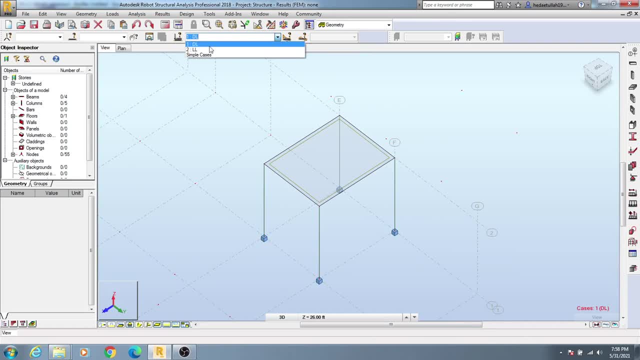 You can see that they have two types of load. I have created dead load and live load only. So if you need to define different types of load, then you are able to define that okay, as per our previous lecture. Now to define load combination, click here loads. Then they have two options: manual combination and automatic combination. In this lecture I'm just going to show that how we'll do about automatic combination. So I'll click here automatic combination And I'll say 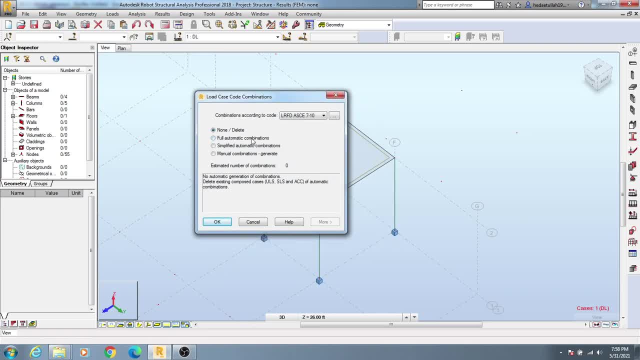 Let's select full automatic combination. I'll select that option And from here you can see that they have different types of code, like ACI 3002, ACI 318, 201 on ASD, LRFD, ASD, ASC 710.. And here, LRFD- ASC 710.. Okay, and 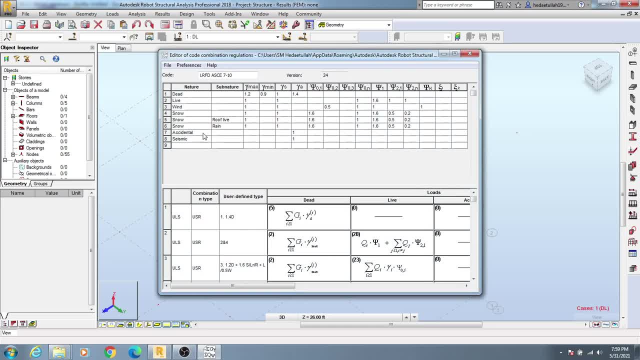 you can click here for different types of combo. okay, so for the dead load here, for live load or for different types of combo, you will see this is here and you can just go down if available, and also you can wash our different types of load combination, okay, so I'll just close that and from here I'll select one of that. 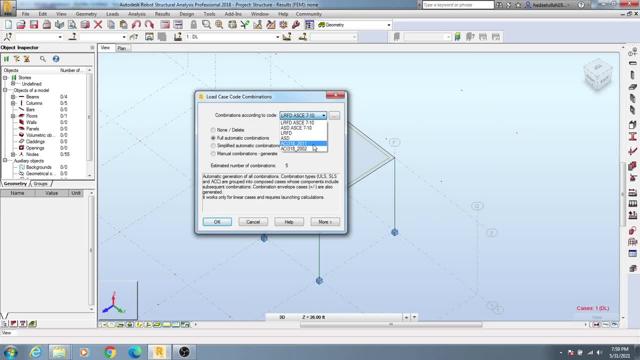 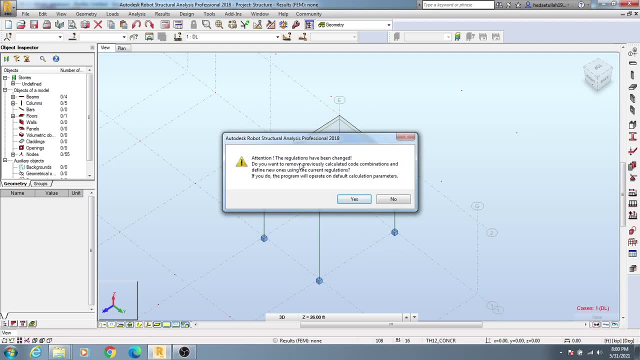 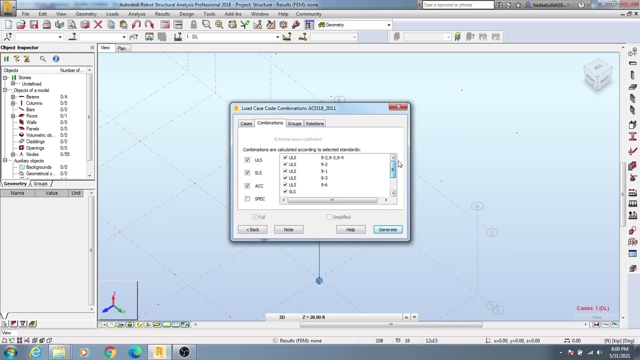 load combinations. I'll select load combo: 3, 1, 8, 2 0, 1, 1. okay, and I'll go okay. yes, you see, here you will see different types of combo. okay, you will see different types of combo, depth, different types of combo and you can use. 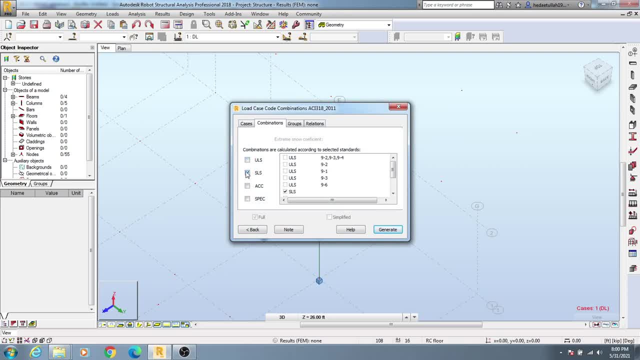 from here as per suitable combination: okay, what will be suitable for a combo you can select from here. okay, now, with the group and the relation. so, and also as the case: 1, 2: okay, so in this way, you are able to defend our combo after the simply click generate and your combo have been created. 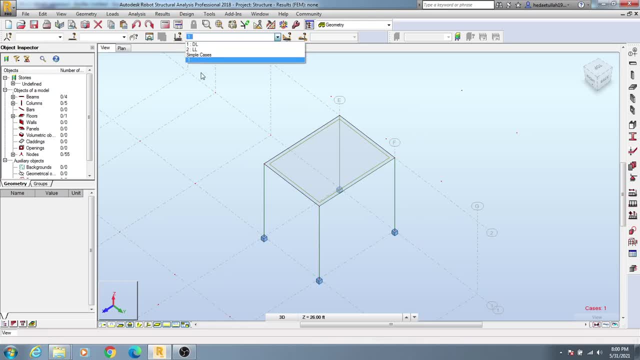 and when you will, just if you click here, okay, when you go for analysis. after that it will be visible to you, okay, so when we'll show you about a full structure or when I'll show you about a full model, then I will try to define that. so thank. 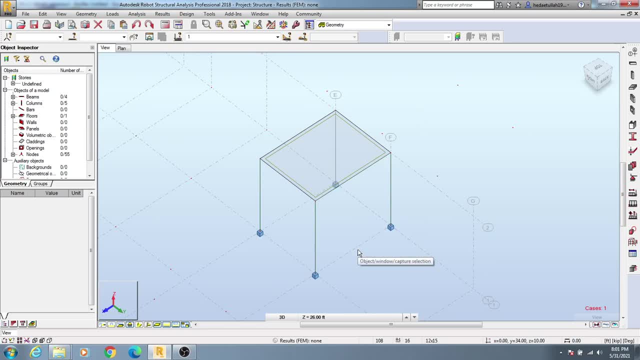 you. thank you very much, sister. stay connected till next video.